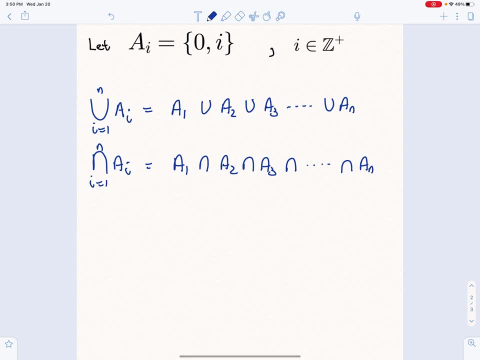 all the way up to an. So it's the intersection of all of those sets. So just to understand where we're coming from with this given set, here we have a sub i is equal to the set 0 and i, where i, is a positive integer. So this means things like a2 is the set 0, 2.. Okay, so let's. 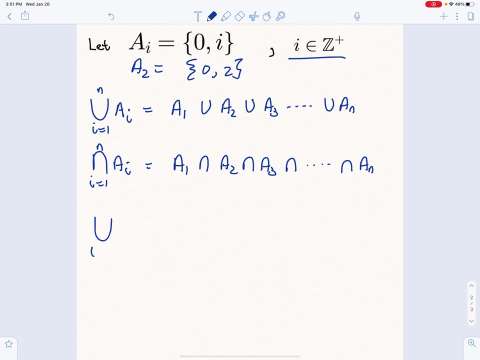 just look at a couple examples. Let's say we want the union. Let's say i going from 1 to 5, of a i in this case. Well, that means we're joining a1,, a2,, a3,, a4, and a5,. 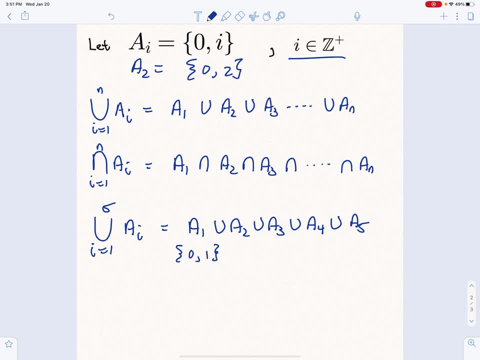 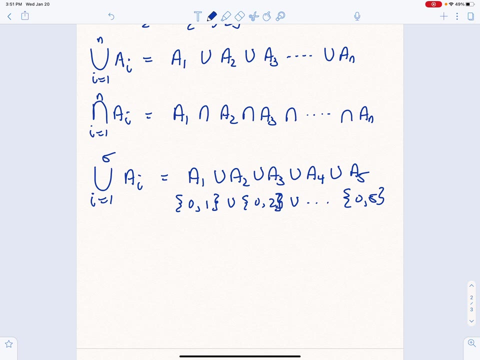 which means we have the set 0, 1 union, 0, 2 union and all the way up to 0, 5.. Now, by looking at those and looking at the patterns, it's easy to see that the union of all of those is going to be the numbers 0 through 5.. 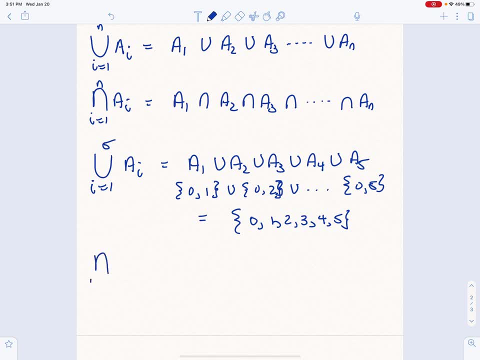 Okay, so how about the intersection of those- And I'm going to say i going from 1 to 5 as well? Well, that's going to be the same thing, except intersection symbols in between them. So what we have to do is look to see if there's 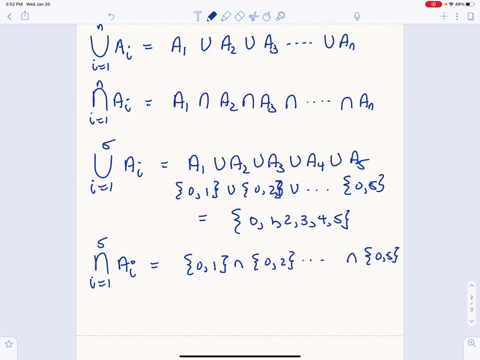 any intersection symbols in between them. So what we have to do is look to see if there's any element common to all of those sets. As it turns out, it sure is. There is one element common to all the sets, and that is the number 0. So the intersection of all of those is the. 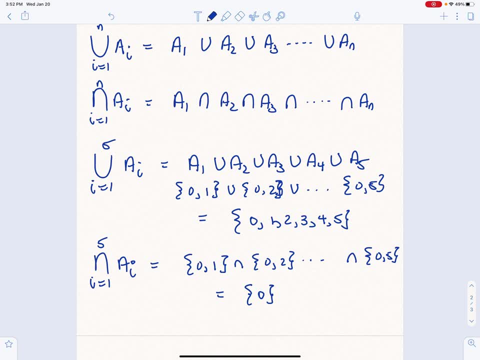 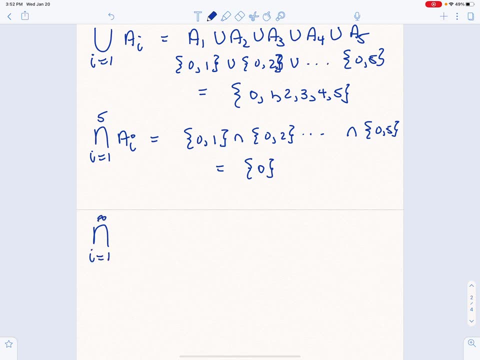 singleton set with 0 in the middle. So one thing we could talk about is going infinite. What if we wanted the infinite intersection of all of those sets? Well, as you can see, every set that's listed is going to contain a 0. So that's going to be the intersection of all of those sets. 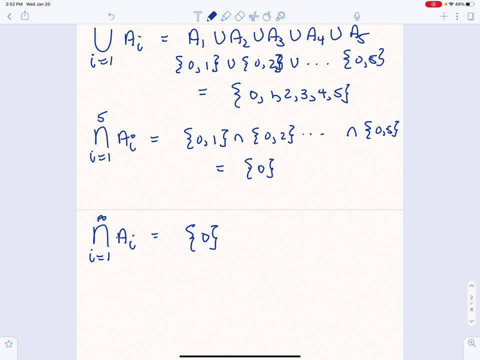 So that means that the intersection is just going to be 0. And the union i, starting at 1 and going to n, would be. well, let's look at those. So up here, I'm going to highlight that for you Up here. 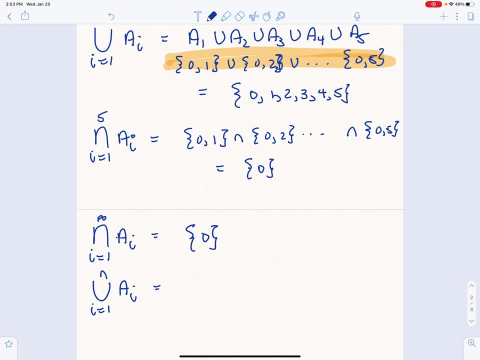 we have the sets 0,, 1,, 0, 2,, 0, 3, etc. So we're going to end up with the set of numbers 0,, 1,, 2,, 3, and onward, and onward, and onward, and never ending.